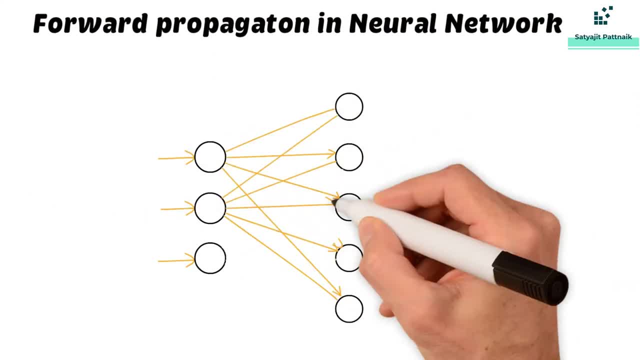 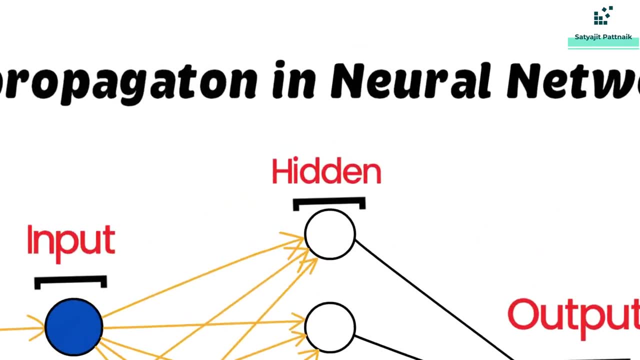 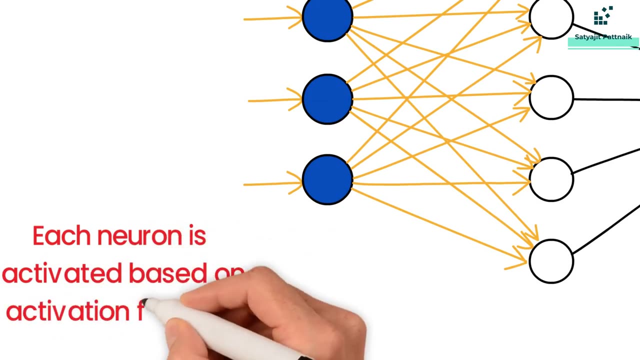 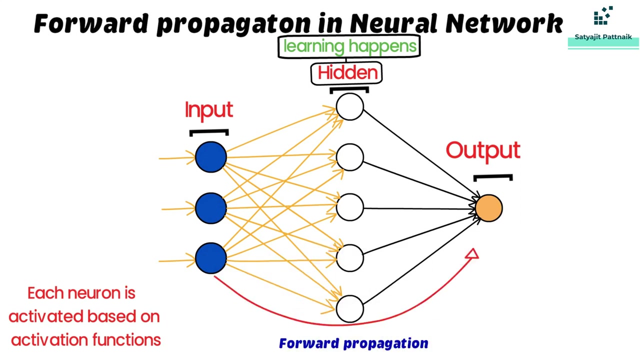 Let's learn about forward propagation in neural network. We have three layers in a neural network: Input, hidden and output. Hidden layer is the layer where the learning happens. Each neuron is activated based on activation functions. Forward propagation is the movement of information from input to the output layer via the hidden. 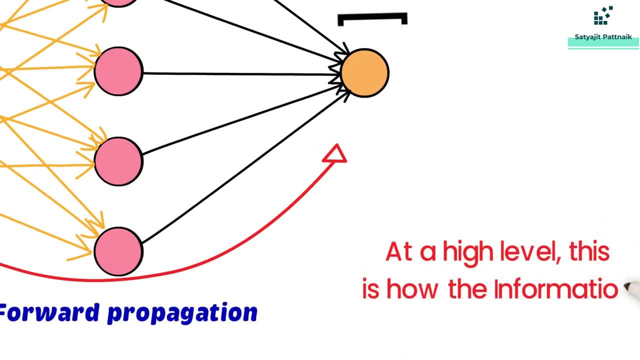 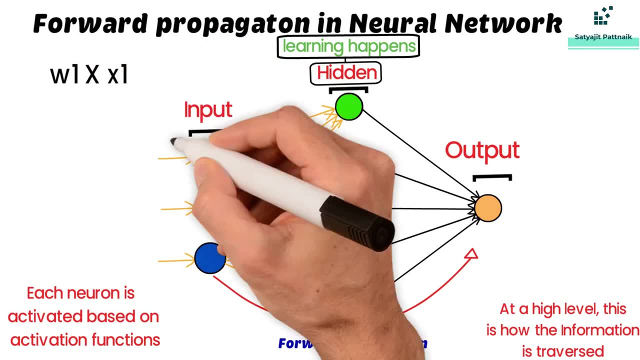 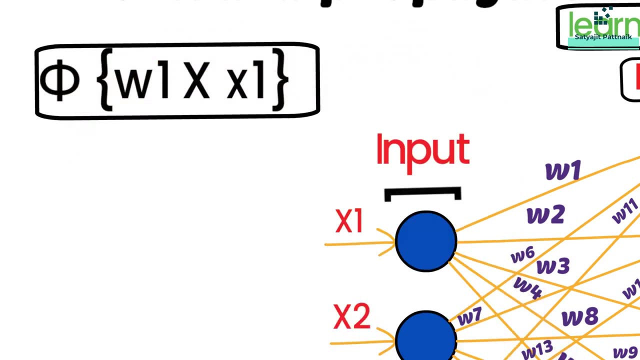 layers At a very high level. this is how the information is traversed. Each neuron in first hidden layer does a dot product of the weight and input they receive. Then this total is fed to an activation function and the output of which goes to the next hidden. 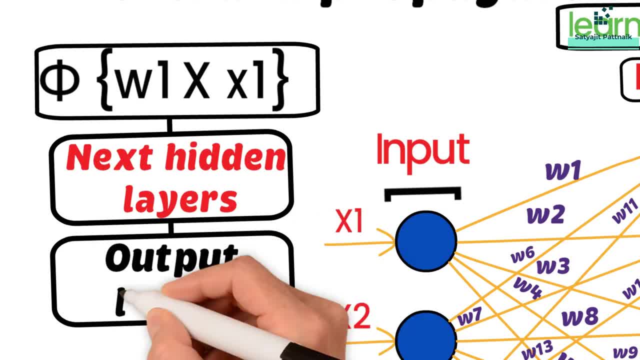 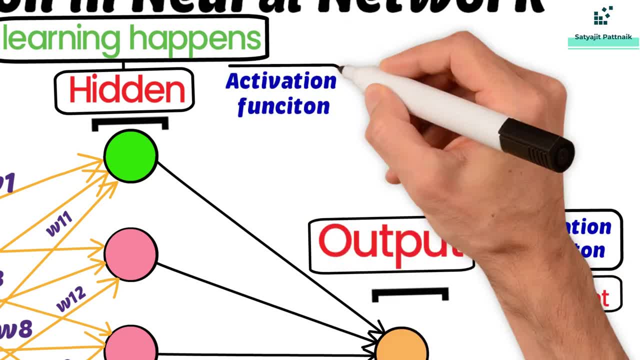 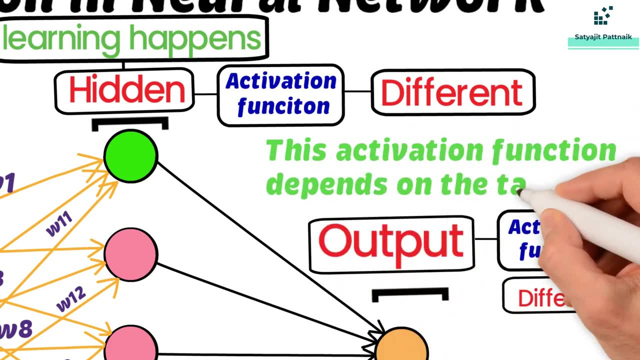 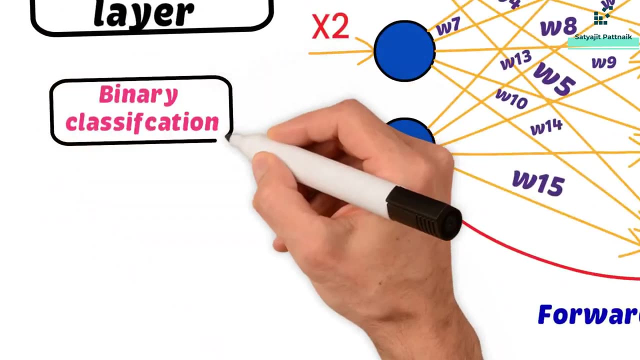 layers This flow repeats until it hits the output layer. In output neuron activation function is different from the activation functions used in the hidden layer neurons. This activation function depends on the task which we are doing. For example, if we are doing a binary classification, we can use a sigmoid function. 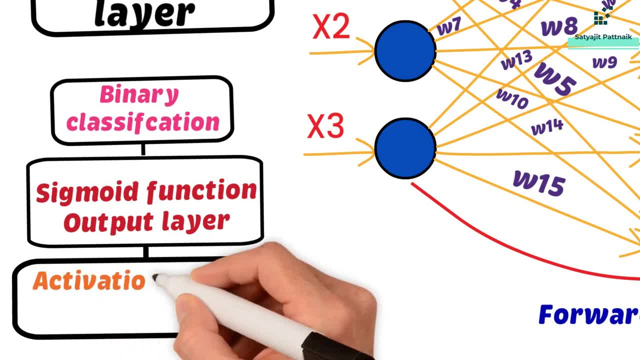 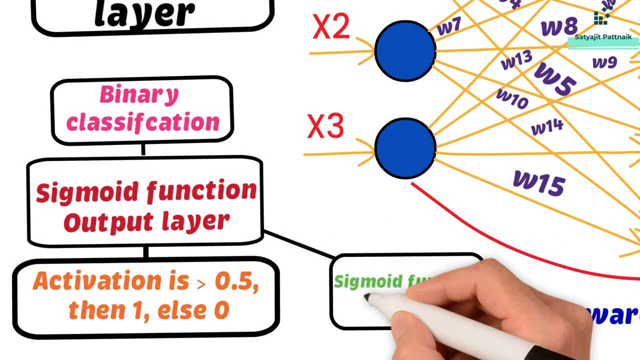 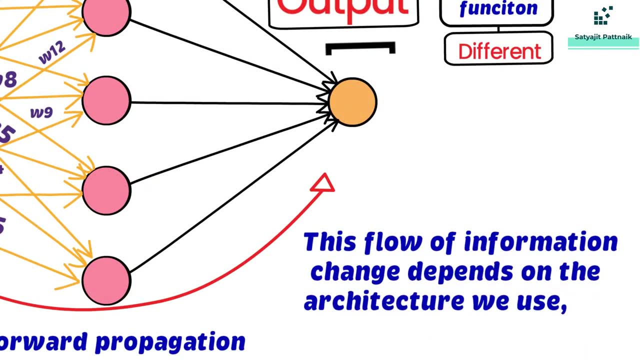 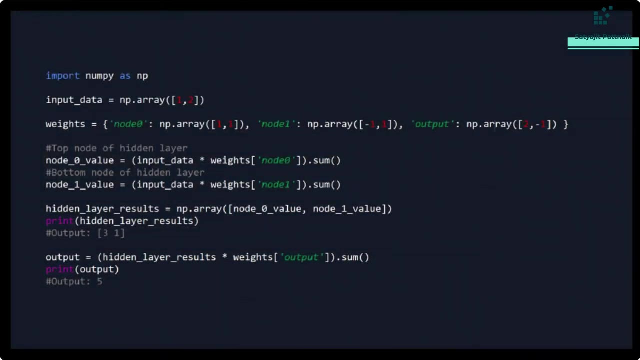 at the output layer. If activation is greater than 0.5, then 1, else 0, because sigmoid function ranges between 0 and 1.. This flow of information change depends on the architecture we use, But the general idea is the same. Let's see how forward propagation works for a single data point. 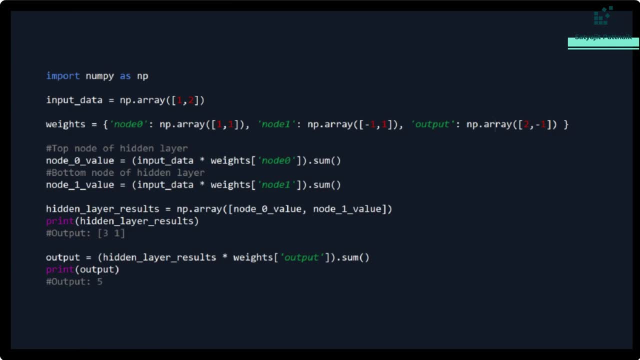 This is a program to understand the concept. We have two nodes of a hidden layer. We have an input which is 1 and 2.. We have defined the weights at each node. node Value at node 0 is basically input data into. 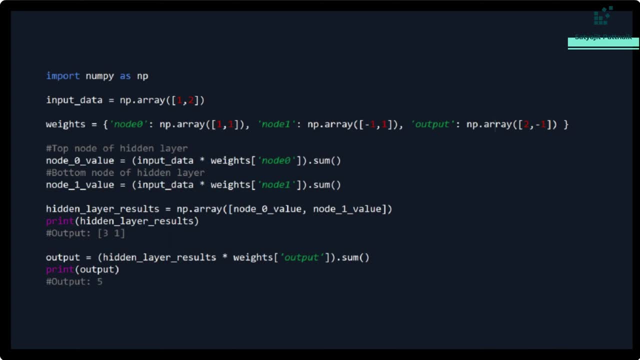 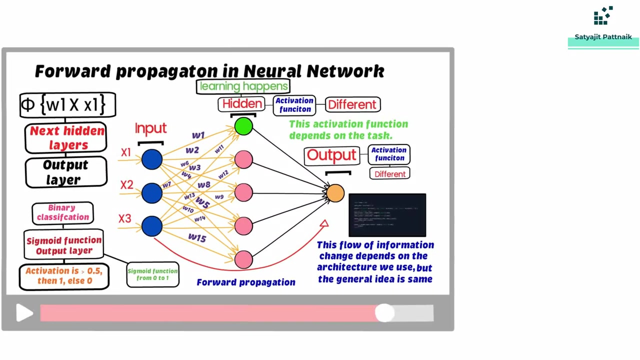 node 0 weights. Similarly, value at node 1 is basically input data multiplied with node 1 weights. Similarly, hidden layer results is done by adding value 1 and value 2 and then it is multiplied with output weights to find the final output. 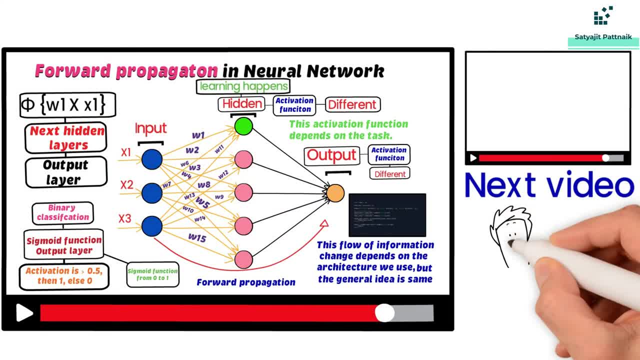 That's all about forward propagation. In the next video we will learn about back propagation in neural networks.